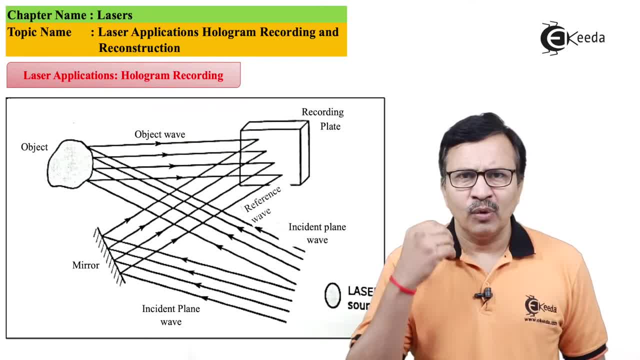 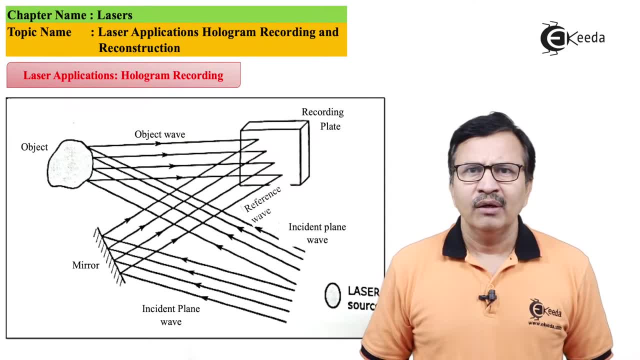 object. So what is the first step in hologram? The first step is nothing but the recording of hologram. For the recording of the hologram we require a very high intensity, coherent and monochromatic source of light. And what can be a better source than lasers? So we use a laser that is very broad. 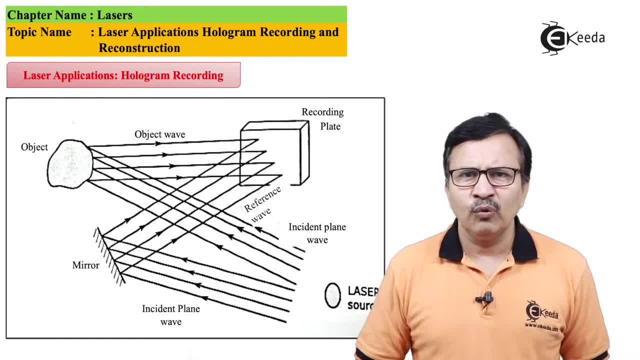 and we split this laser into two rays. One of the rays is the reference beam and the second ray is actually called as the object beam. So the reference beam is made to fall on a mirror, whereas the object beam is actually made to fall on the object. 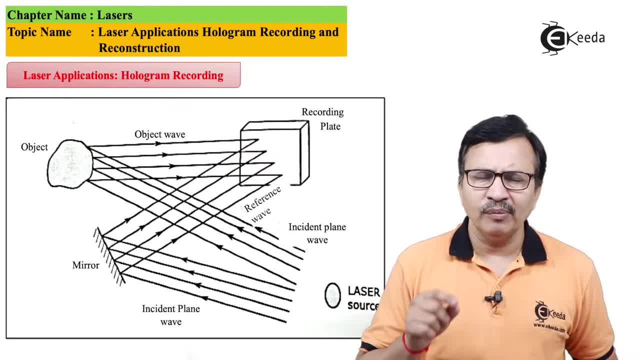 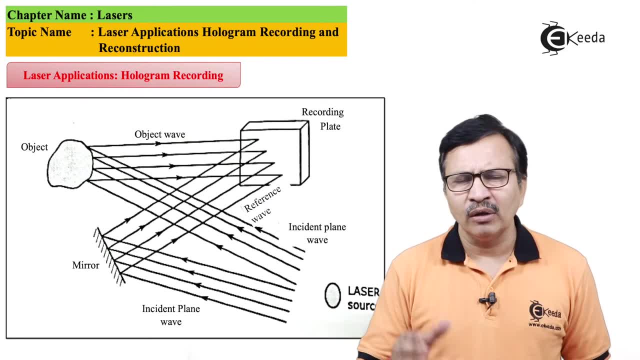 So the reflected beam from the mirror, which is basically the reference beam, will actually be incident on a photographic plate and simultaneously the object wave will also be incident on the same photographic plate. So when we are having these two waves, one is the object wave and the second is the reference. 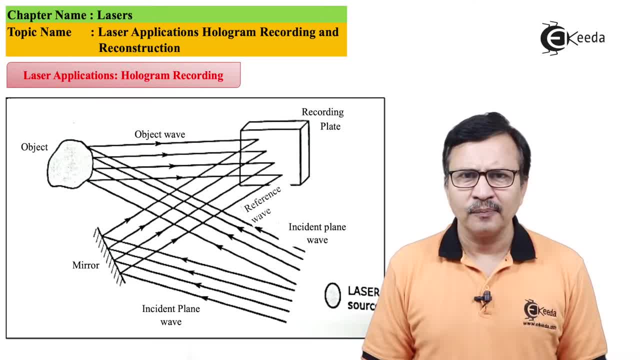 wave. both these waves will actually interfere, But when they are interfering they will actually capture the phase of the object, And this phase and the intensity will actually be recorded as an intensity pattern on the photographic plate. This is how we record a hologram In the second part. 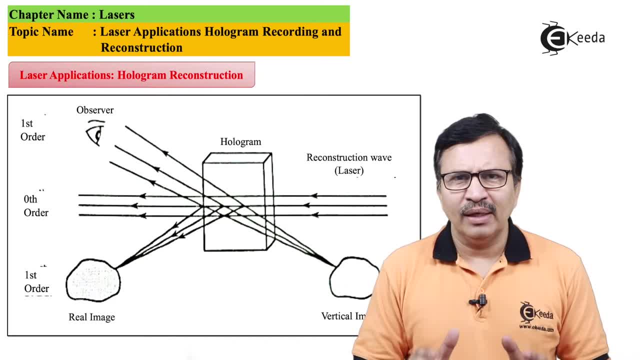 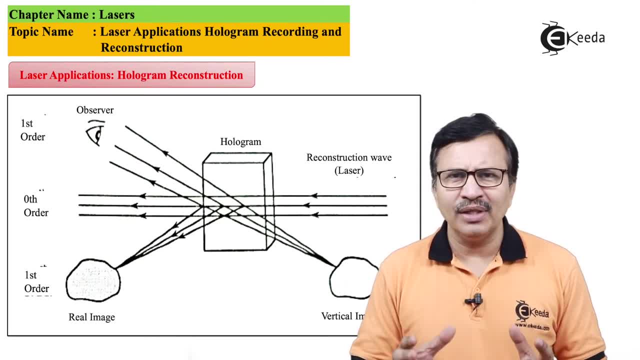 In the second part we deal with how to read this hologram. In the second part we deal with how to read this hologram. of the hologram, we actually use the same wavelength of light that was actually used for the recording purpose. By light I mean over here the laser light. and when this particular